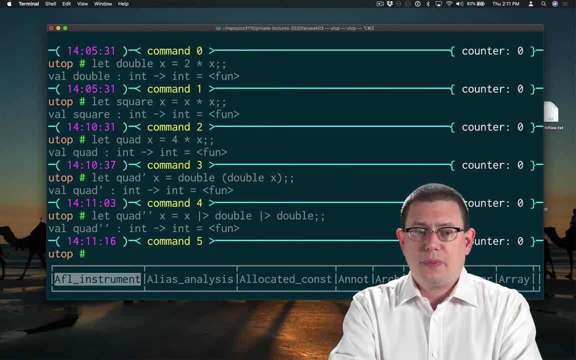 So that's a bunch of different ways of writing quad. Now suppose you wanted to take the fourth power of a number. I don't really know what that would be in terms of squaring, but let's call it fourth, Let's see. 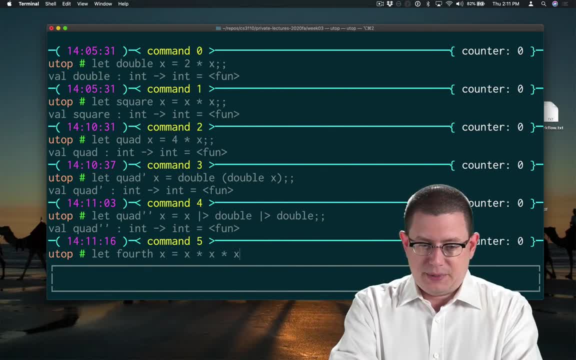 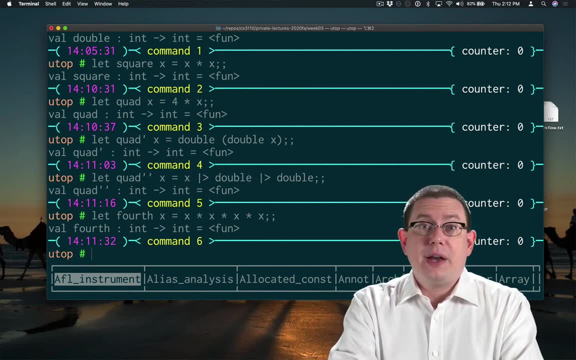 Fourth of x could be x times x times x times x. This is kind of similar to quad. We could also write it, rewrite it. that is in the same way as we rewrote quad. So we could have let fourth prime of x be the result of taking quad. 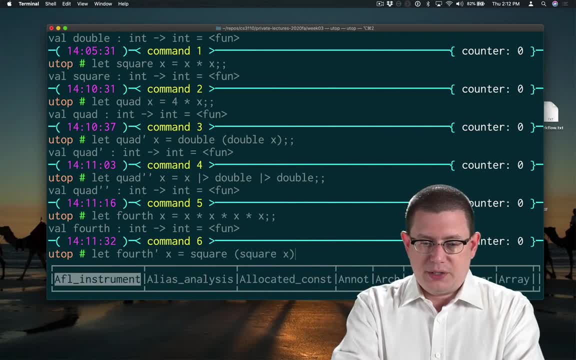 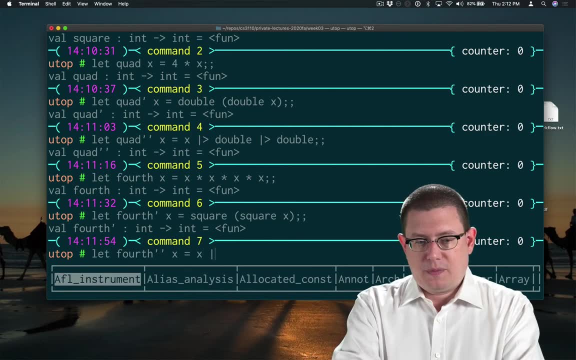 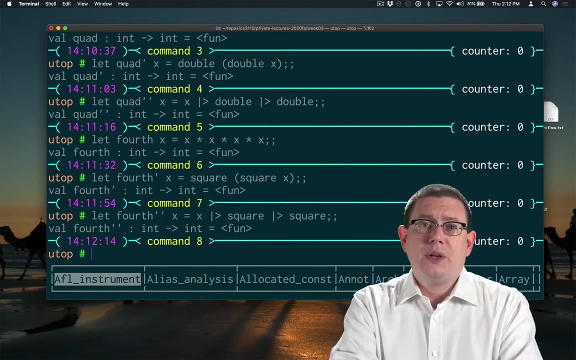 or square rather, and applying square twice to the argument. Or we could do it with a pipeline operator. So that gives us a bunch of different ways of writing the same function. Now, those were not maybe that interesting of functions, but let's look at the similarity between what we did for each of them. 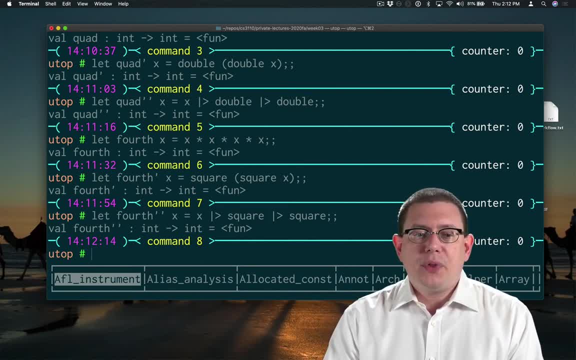 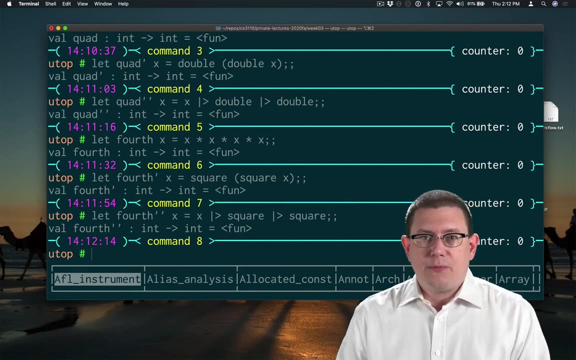 In order to build quad, we applied double twice. In order to build fourth, we applied square twice. So there's this notion here of applying a function twice. Well, anytime you notice that kind of repeated action in a code, a good question to ask yourself is: 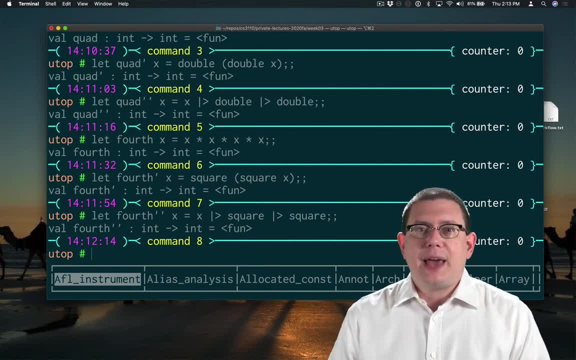 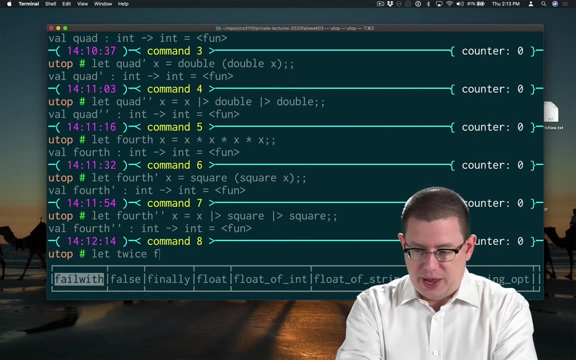 could I factor that out? Could I abstract that functionality and make it its own piece of code so that I don't have to keep repeating it? So let's write a function that actually applies another function twice. Twice will take in a function f and an argument x. 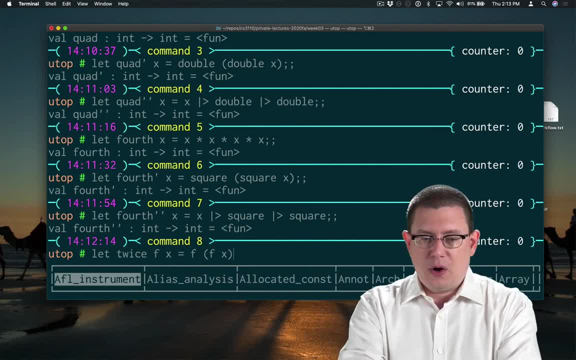 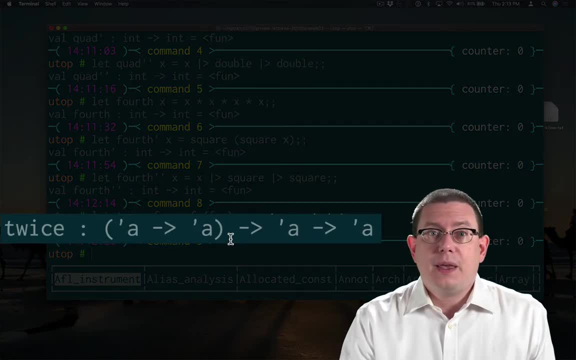 and it will apply f to that argument twice. Let's look at the type of that function. Twice takes in a function, a function, from alpha to alpha, So it doesn't really matter what the input-output type of that function is. It could be anything. 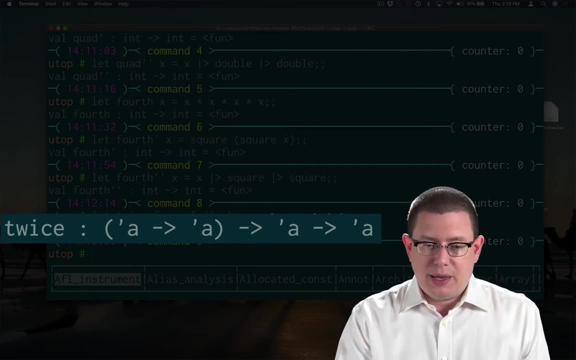 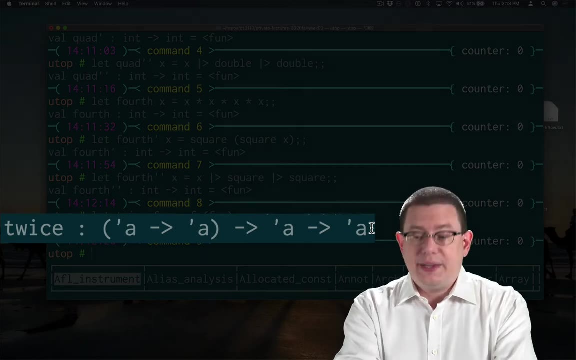 It then takes in a value of the input type and gives us back a value of that type, which is also the same as the output type of the function. So I could use twice to recode some of the functions that I wrote before. For example, I could write quad: 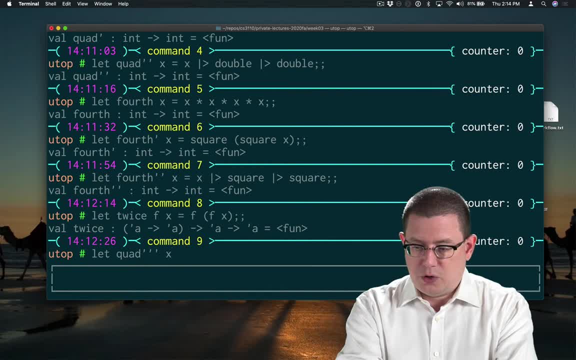 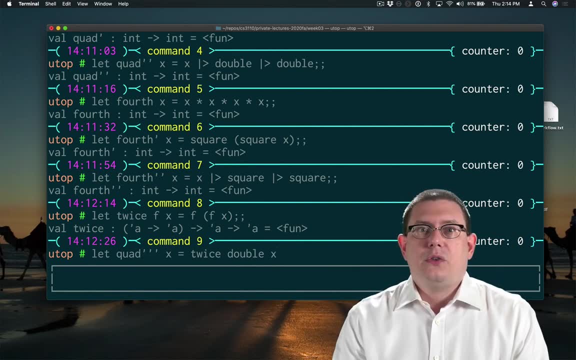 Let's see what are we up to. Triple prime here. Quad of x could be twice double x, So I'm going to take the double function and apply it twice to x. This is higher order. We're actually using twice as a function. 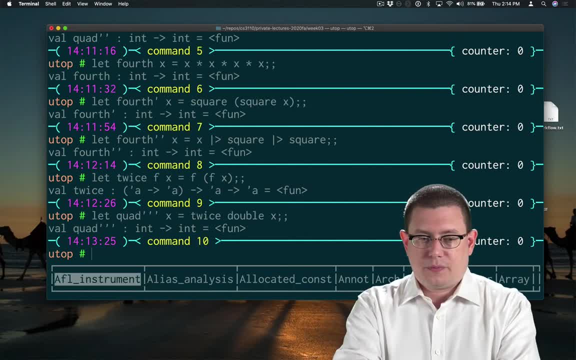 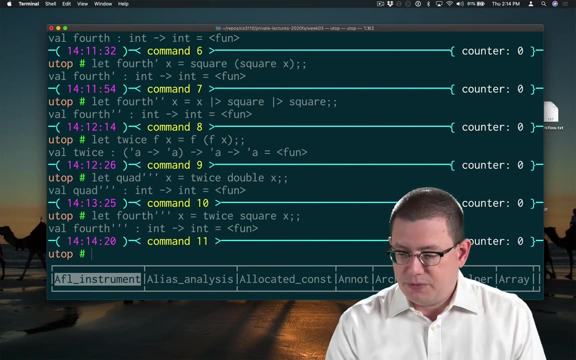 that takes in another function as an argument. I could do the same thing with fourth. So let's see, let fourth triple prime be twice square x, And of course I could have done all of that with twice, using the pipeline operator as well. 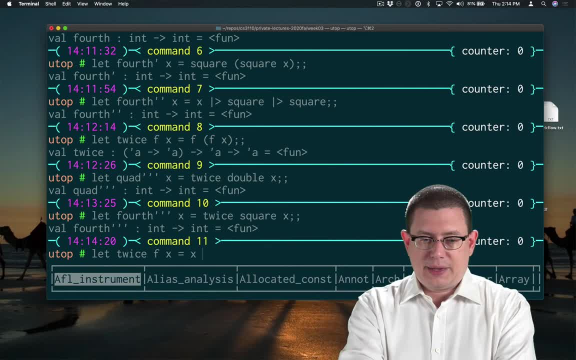 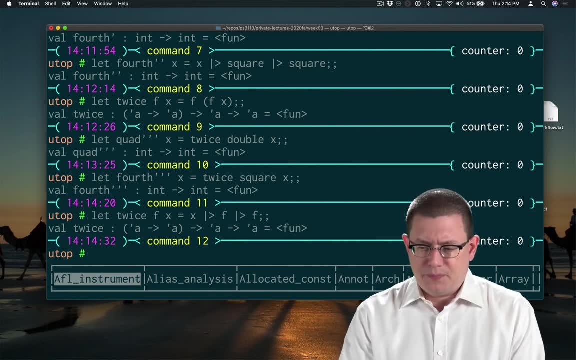 I could have written it as f x equal x, pipeline through f twice. That would work just as well. I won't go back and rewrite the other functions with that, but you get the idea. Another thing I could do for quad and fourth is actually leave off the argument. 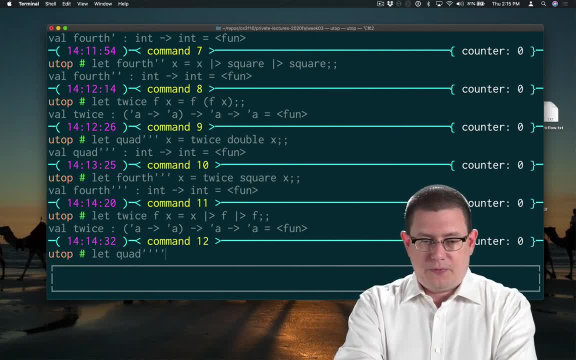 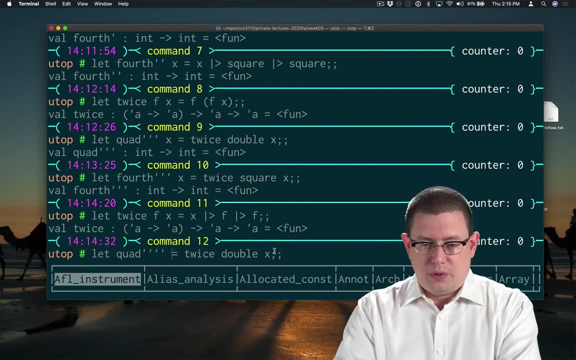 I could rewrite quad- we're up to four primes here- as twice double x, If I leave off the argument. what I mean is suppose I just said quad were this, in which quad is not taking in an argument here, but it is equal to twice double. 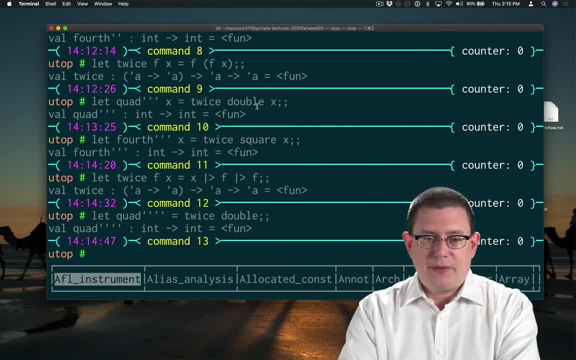 So what's twice double? Well, twice. we can see the type of it up at the top here: takes in a function, takes in an argument, gives us back an output. But if we apply twice only to its function, f in this case, we did twice double. 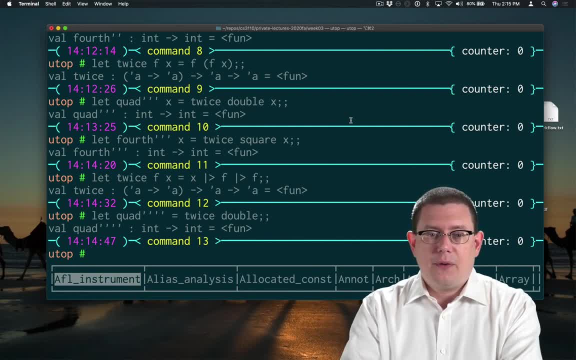 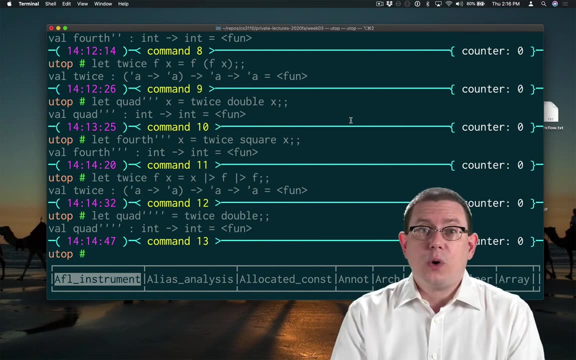 what that gives us back is a function, A function of type alpha- arrow alpha. or, in this case, since double was defined based on integers, a function of type int- arrow int. So, again, this is higher orderness. Twice, here is being a higher order function.